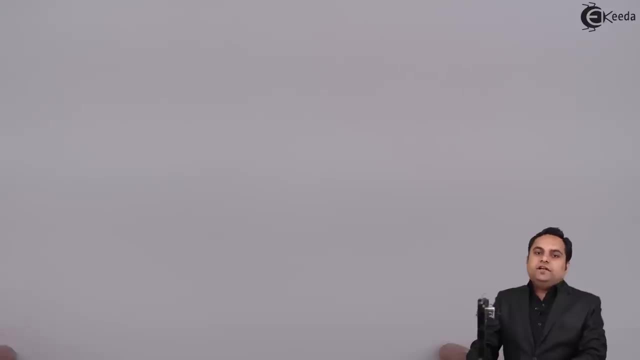 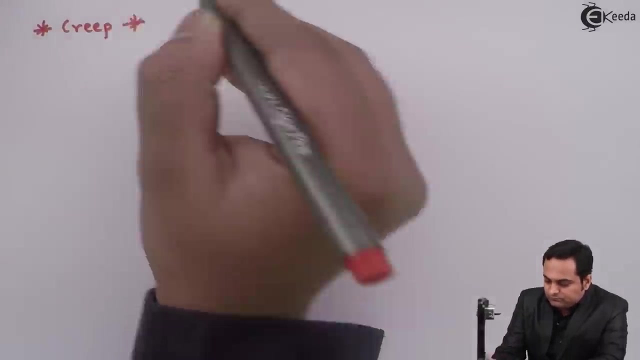 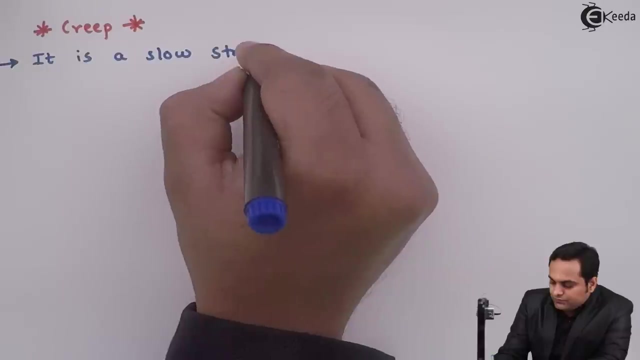 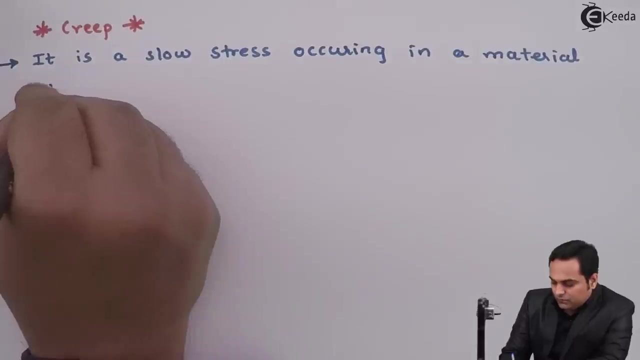 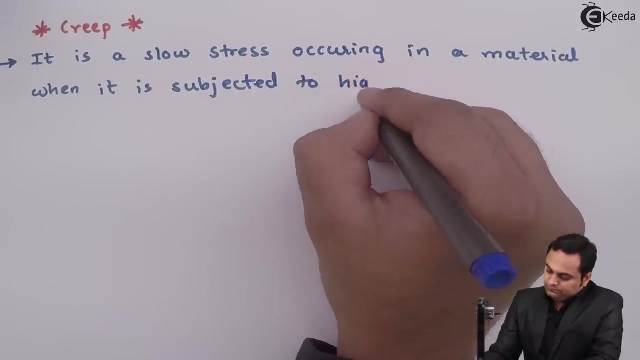 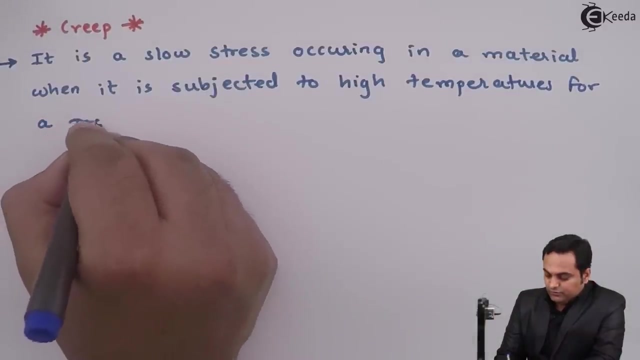 Hello friends, here in this video we are going to see what is meant by creep. Let us get started with the definition first. Creep, it is a slow stress occurring in a material when it is subjected to high temperatures for a prolonged period of time. 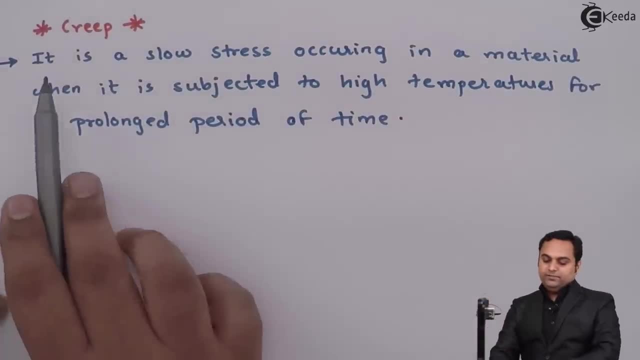 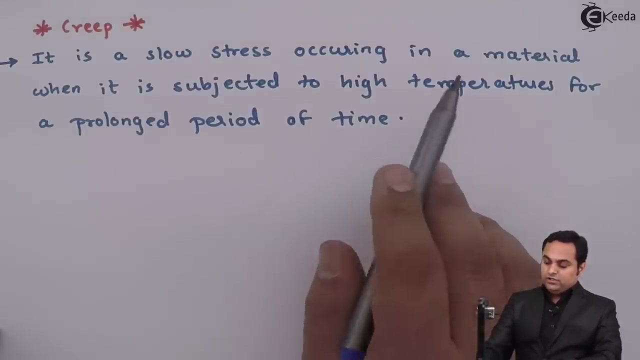 So here I have written the definition of creep. That creep it is a slow stress. We can say the value of stress will occur after many attempts, because it is not an instant stress, It will take time. So it is a slow stress occurring inside a material. 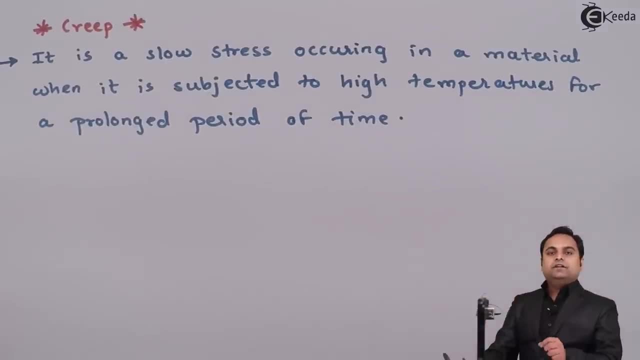 when it is subjected to high temperatures. That is, for creep the condition should be: a material should be subjected to high amount of stresses which are at high temperatures. So creep is basically related to temperature. So if a material is subjected to high or low temperature, 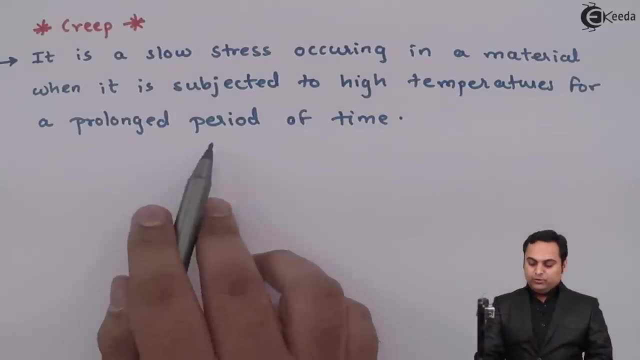 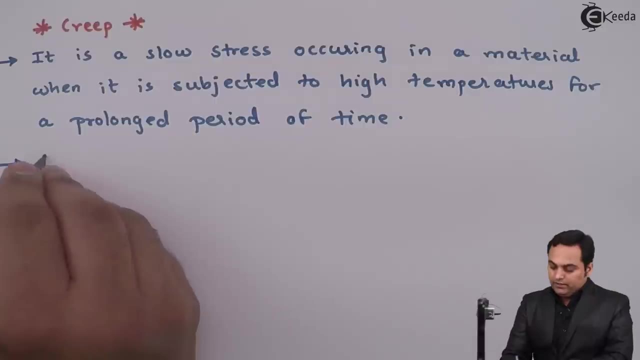 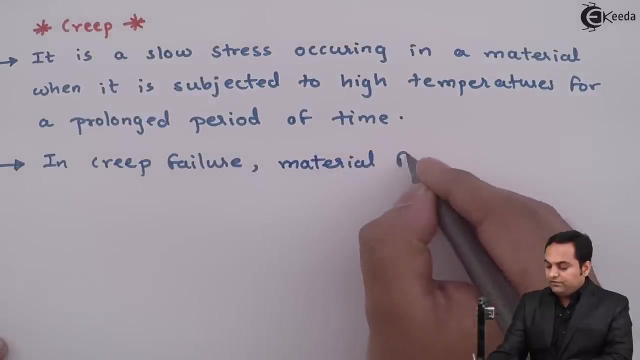 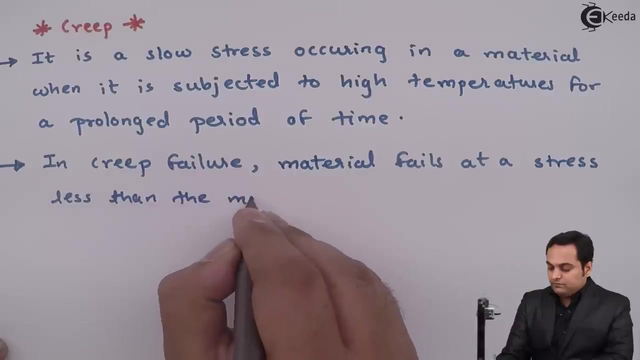 then that material has creep For a prolonged period of time. for a prolonged period of time, and even the duration of creep should be long. Next in creep failure, material fails at a stress less than the maximum stress. So when we are considering creep, 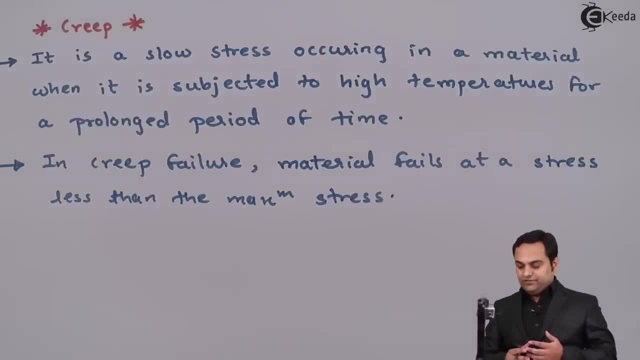 that is a material which is subjected to high temperatures, for example, then because of that high temperatures over a long period of time- stresses are induced or stored inside the material, and when we are applying a load value which is less than the maximum load, then the material fails. 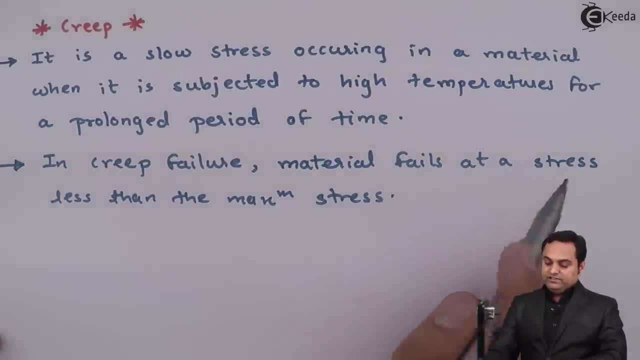 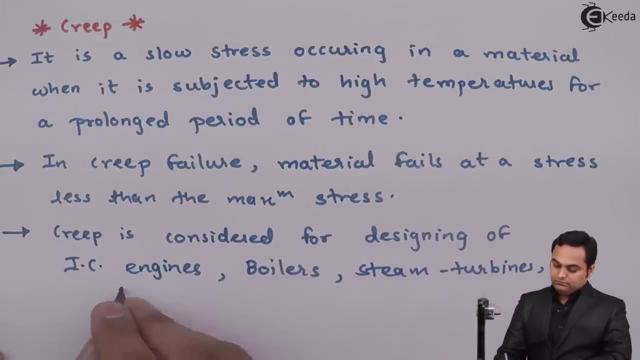 It is called as creep, So it will fail at a stress value which is less than the maximum stress. Next creep is considered for designing of IC engines, boilers, steam turbines, gas turbines, etc. So these are the components which are subjected to high temperatures. for designing such components. we are considering creep. Next. creep is also associated with high temperature, also a permanent deformation. that is, when the material fails because of creep. the material gets permanently deformed, the shape changes and it cannot return back to its original position. so creep is also a permanent deformation. next,